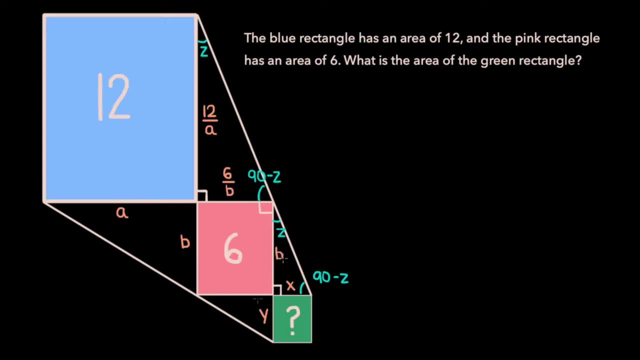 sides of the pink rectangle. We know the longer side is of length b and that the shorter side is of length 6 over b. Now, since these two triangles are similar, we know the ratio of the sides opposite the angle z in both triangles. so 6 over b over x must equal the ratio of the sides. 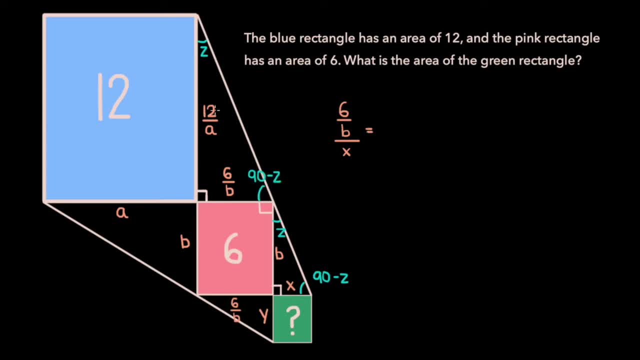 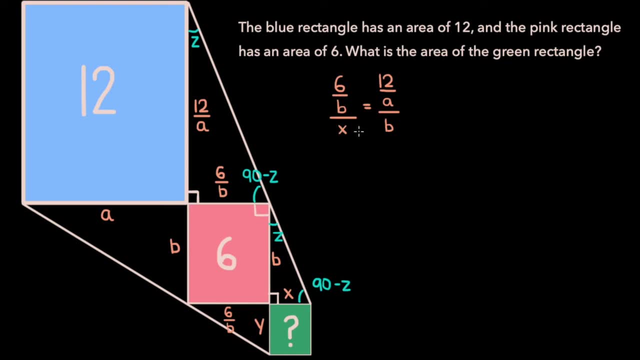 opposite the angle, 90 minus z in both triangles, so 12 over a over b. Now if we cross multiply we get 12 over a times x. so 12x over a equals 6 over b times b, so 6.. Now to isolate x we're going to multiply both sides of this equation by a. 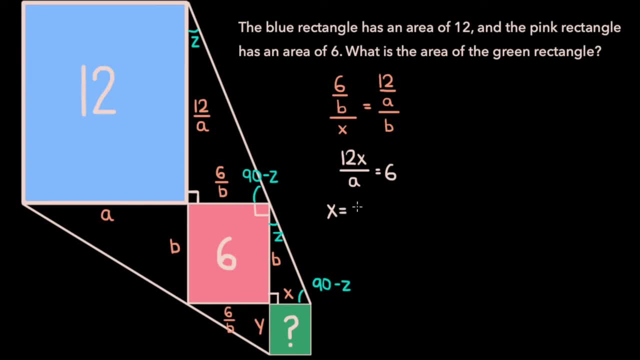 and divide both sides by 12.. And if we do that, we're left with: x is equal to 6a over 12, which simplifies to a over 2.. Now we can do essentially the same thing for y, it turns out. 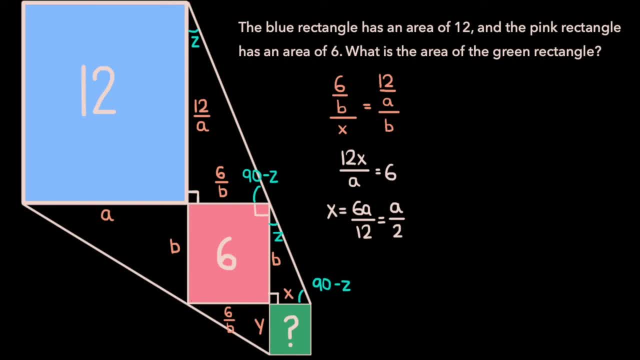 that this triangle and this triangle are similar. I'm not going to go through the same step-by-step process of showing that each of the angles in these triangles are the same, but if you were to, you would find that this angle and this angle are the same and that this angle and this angle. 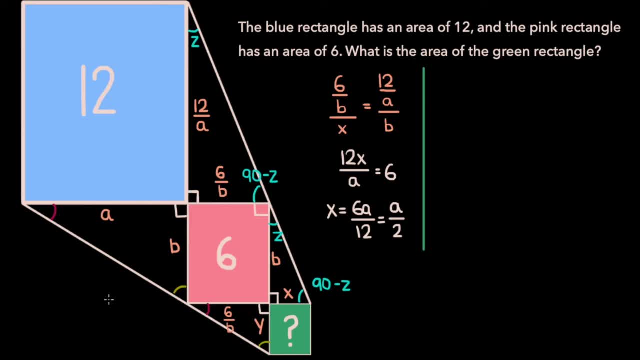 are also the same Because these two triangles are similar. we know the ratio of the sides opposite the yellow angles in these two triangles, so a over 6 over b must equal the ratio of the sides opposite the red angles in these two triangles, so b over y. Now once again we can cross multiply. 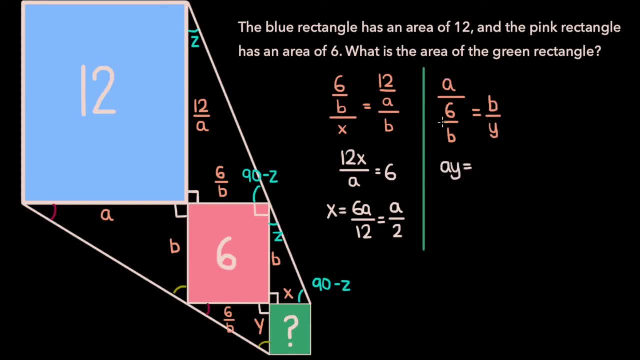 a times y is equal to b times 6 over b, which is just 6.. To isolate y, we can divide by a on both sides and we get y is equal to 6 over a. Now recall that we're looking for the area of the green rectangle, which is just x times y. 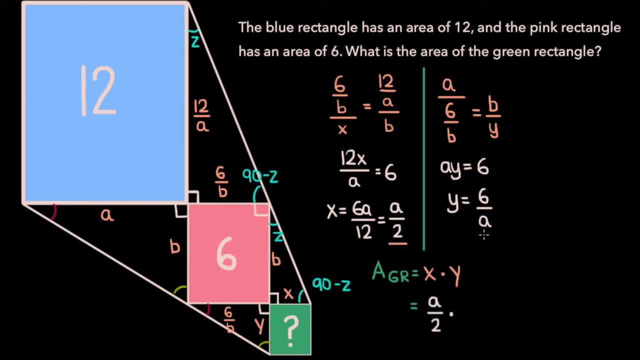 x is a over 2, and y is 6 over a, so the area of the green rectangle is a over 2 times 6 over a. We can cancel out the a in the numerator with the a in the denominator and we're left with the area. 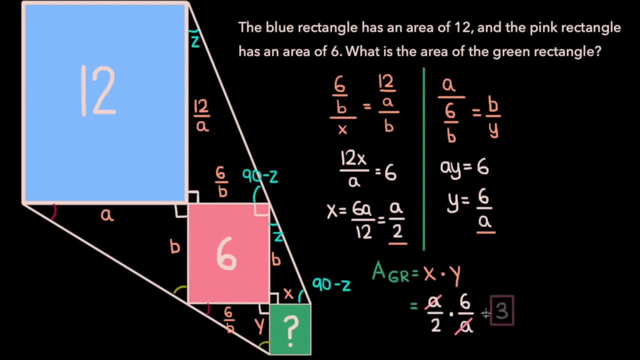 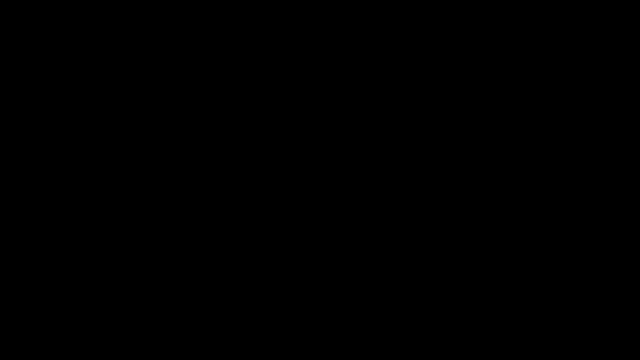 of the green rectangle as 6 over 2, which is 3, and that's all there is to this problem. Alright, so that about wraps it up for this video. if you enjoyed it, leave it a like, and if you want to be notified when I post more content like this, make sure to subscribe. Thanks for watching.